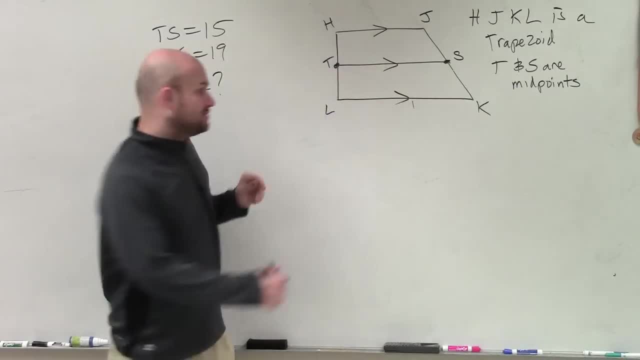 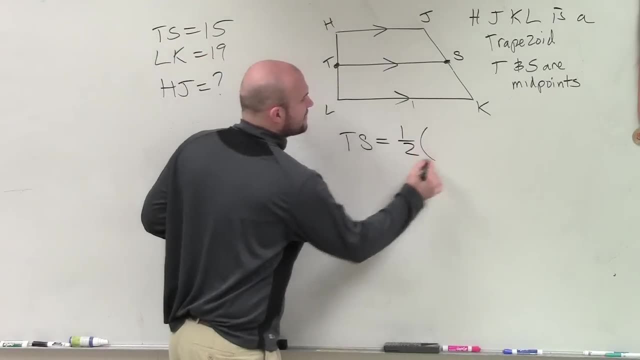 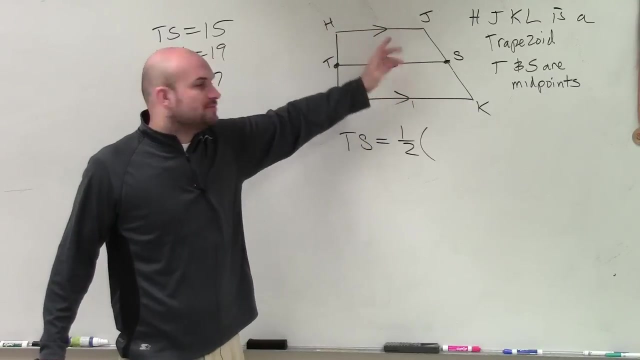 is if I wanted to find the measurement of TS, which is your midsegment right? Remember the midsegment. It was equal to 1 half your base plus your other base, right? Remember you added your two bases, multiplied them 1 half. 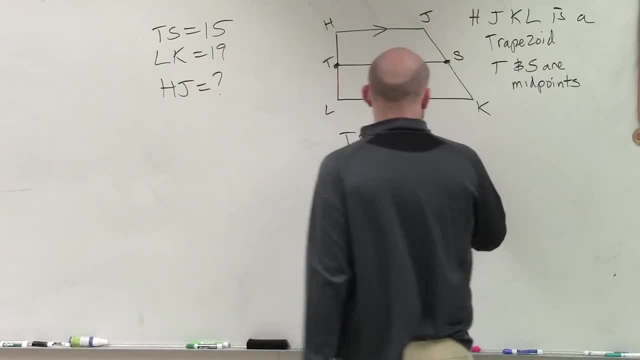 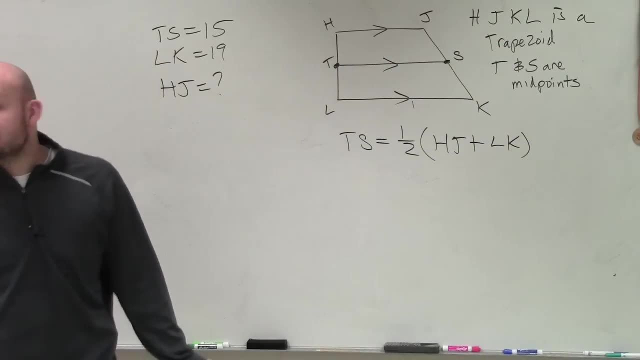 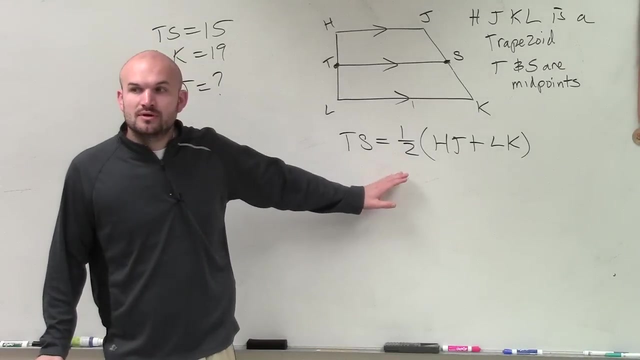 That gives you the length of the midsegment. So this is HJ plus LK. That's the formula for the midsegment theorem. We did it for a different trapezoid. But the main important thing is your midsegment is equal to half. 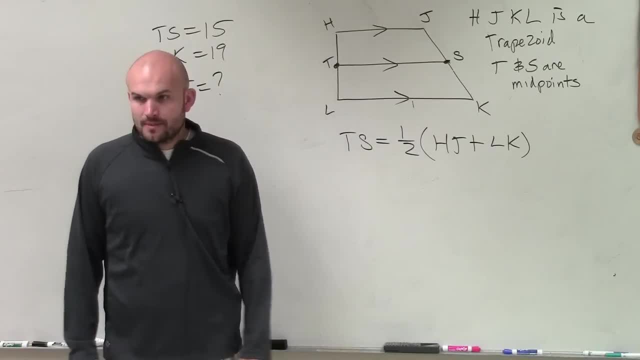 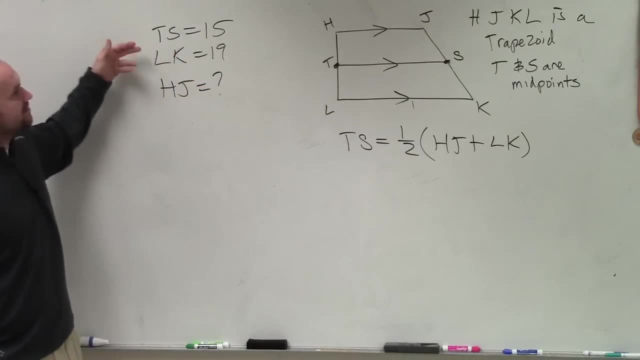 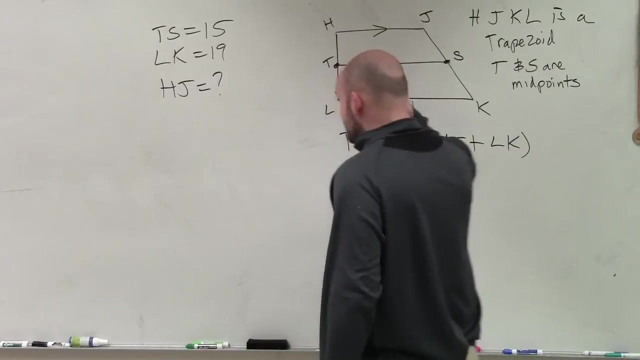 of the sum Of your two bases. All right, But in this problem, do we know what the midsegment already is? What's the length of our midsegment 15.. And then, what is one of our bases? Well, we don't know what HJ is. 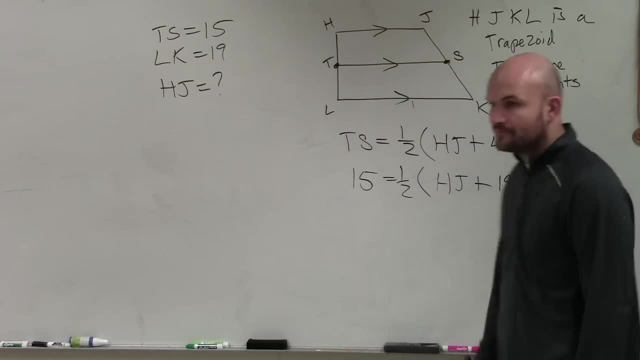 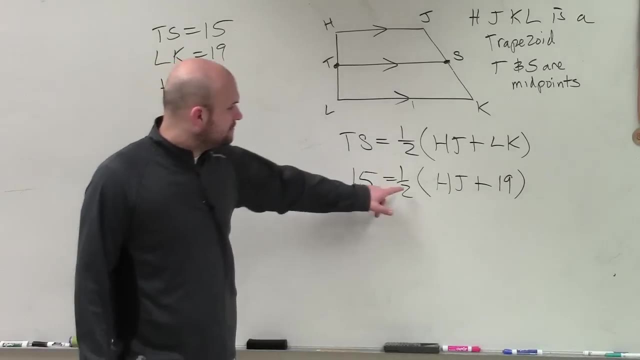 Plus, do we know what LK is There? we go All right. So now we need to say, all right, how do we solve for HJ? Well, right now, guys, We're, right now, we're multiplying this parentheses. 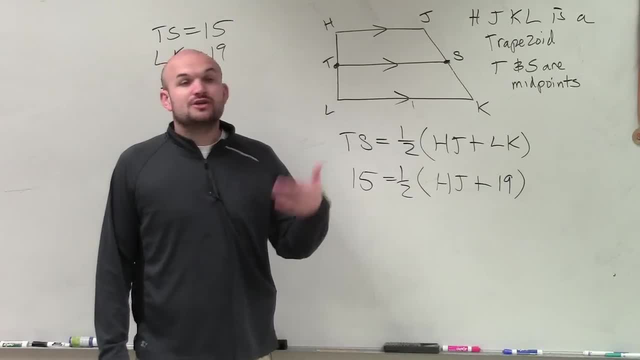 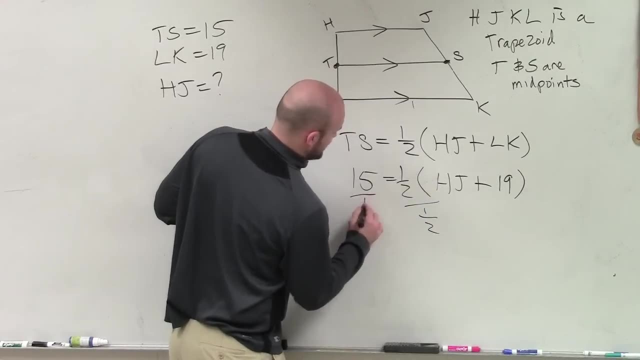 as being multiplied by 1 half, right. So to undo multiplying by 1 half, you can do what: Divide by 1 half, And you guys might say, oh jeez, I don't want to divide fractions. Does anybody remember what you do when you divide a fraction? 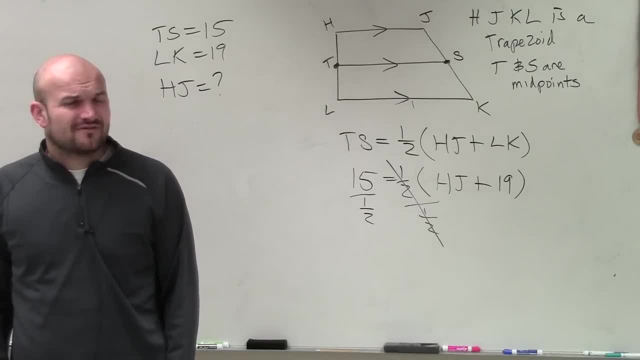 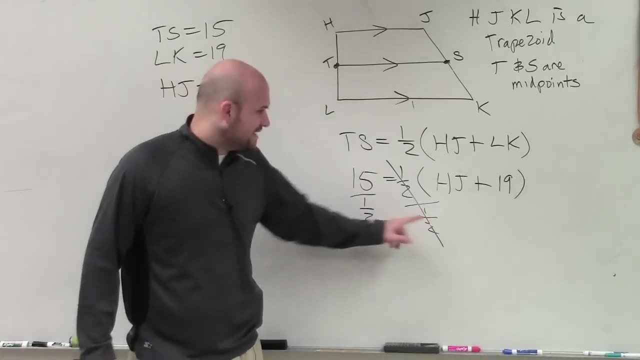 How do we actually divide fractions? Does everybody remember? We don't really like dividing fractions, We use a different operation. Yes, Megan, We multiply by 1 half. Well, yeah, Well, we did that. You can multiply 1 half by both sides. 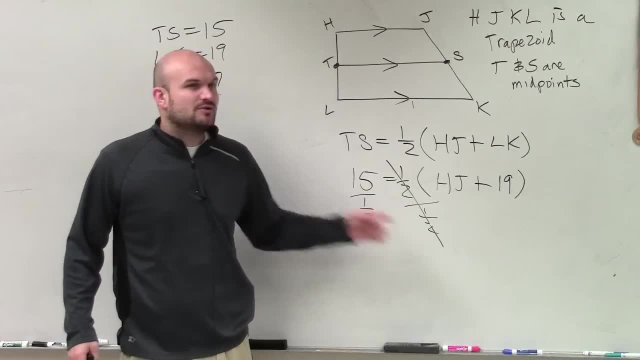 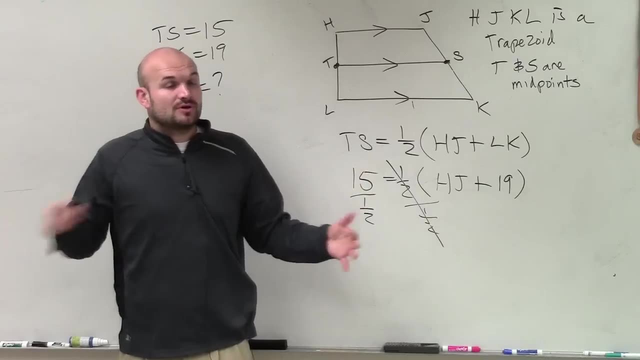 That's the same thing as dividing by both sides, But you don't want to multiply both sides by 1 half. You want to multiply by a different type of the number or a different way: By the reciprocal, By the reciprocal. So what I did last class period is yes. 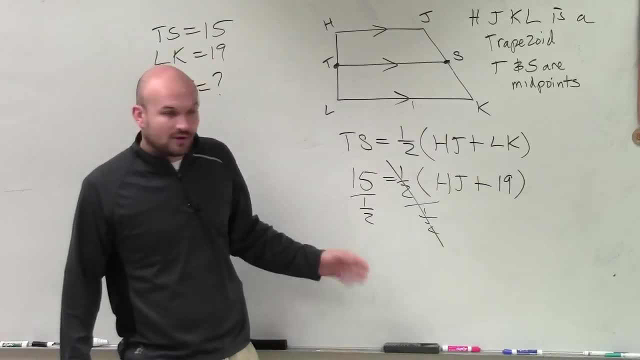 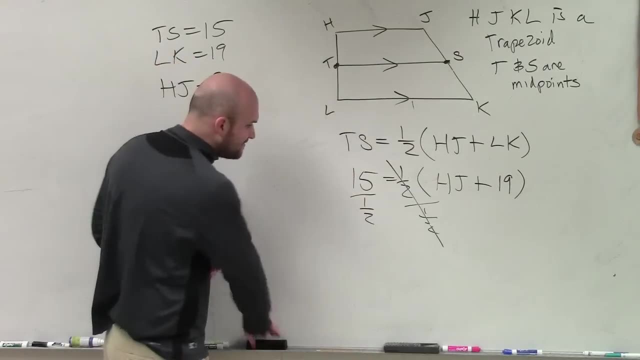 instead of having 1 half, you can multiply both sides by the reciprocal. In this problem, what I did is I divide, But instead of taking 15 divided by 1 half, 15 divided by 1 half is the same thing.